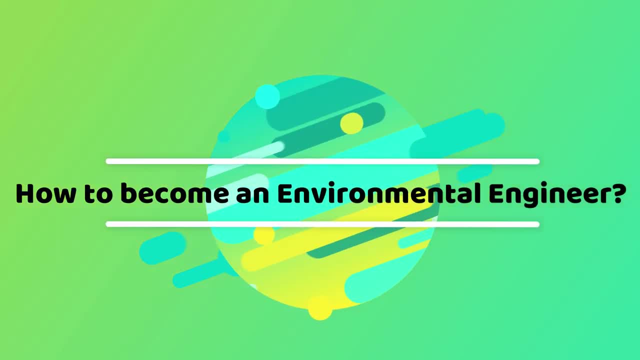 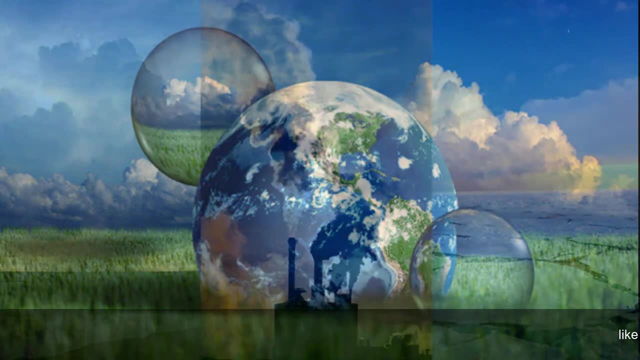 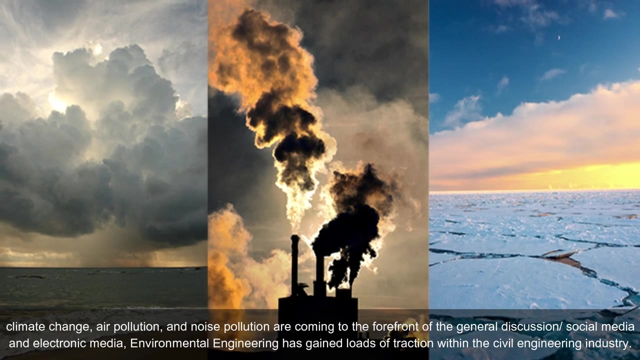 How to become an environmental engineer. Environmental engineering is not a very branded discipline to the newbie civil engineers, but as the issues like climate change, air pollution and noise pollution are coming to the forefront of the general discussion- slash social media and electronic media- environmental engineering has gained loads. 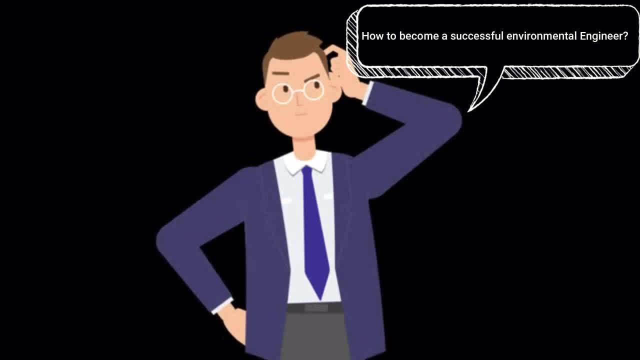 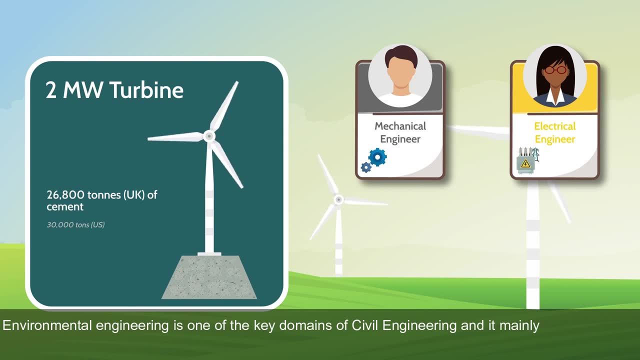 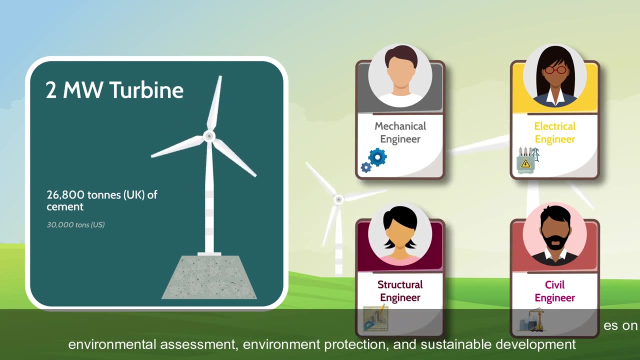 of traction within the civil engineering industry. So how to become a successful environmental engineer? What is environment engineering? Environmental engineering is one of the key domains of civil engineering and it mainly emphasizes on environmental assessment, environment protection and sustainable development. In today's day and time, 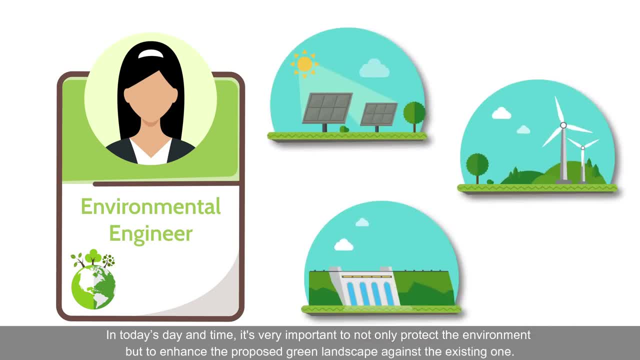 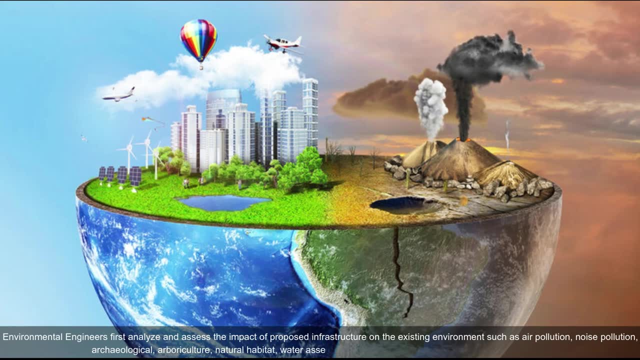 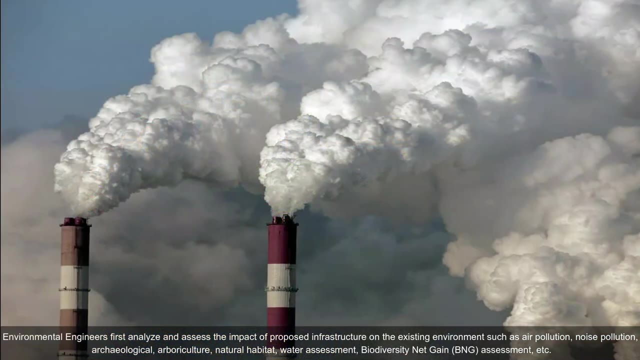 it's very important to not only protect the environment but to enhance the proposed green landscape against the existing one. Environmental engineers first analyze and assess the impact of proposed infrastructure on the existing environment, such as air pollution, noise pollution, archeological arboriculture, natural habitat, water assessment, biodiversity. 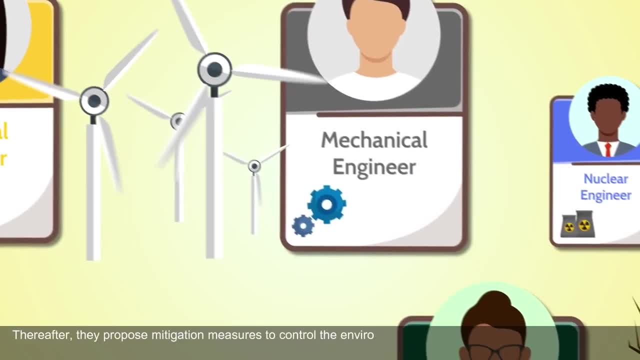 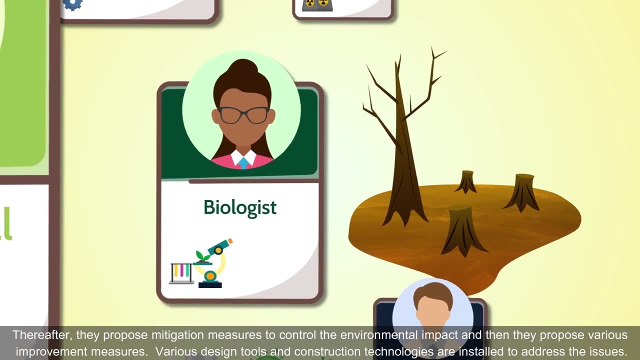 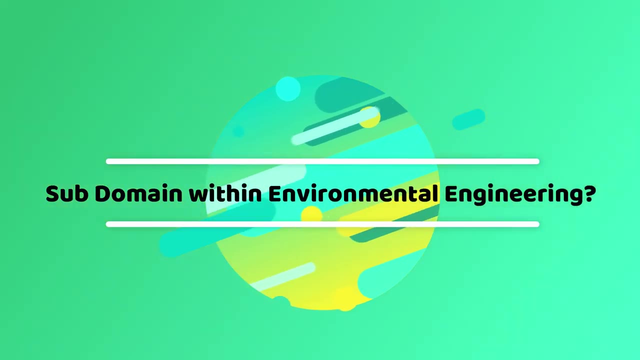 net gain assessment, etc. Thereafter they propose mitigation measures to control the environmental impact, and then they propose various improvement measures. Various design tools and construction technologies are installed to address the issues Subdomain within environmental engineering: Air quality, Noise assessment, Water quality. 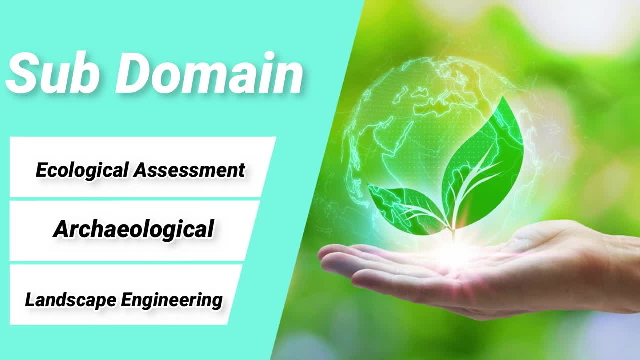 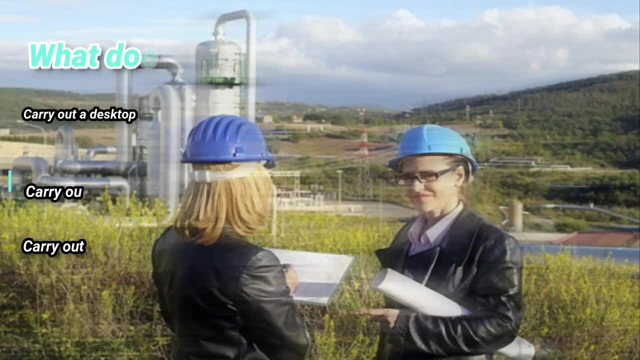 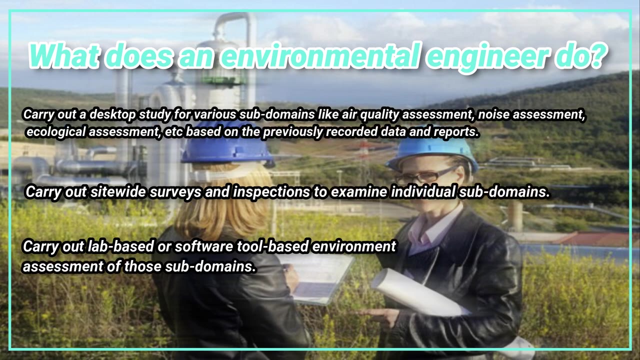 assessment, Ecological assessment, Archaeological, Landscape engineering. What does an environmental engineer do? Carry out a desktop study for various subdomains like air quality assessment, noise assessment, ecological assessment, etc. based on the previously recorded data and reports. Carry out site-wide surveys and inspections to examine individual subdomains. 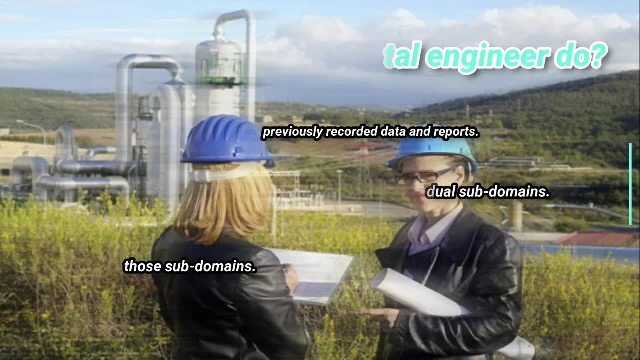 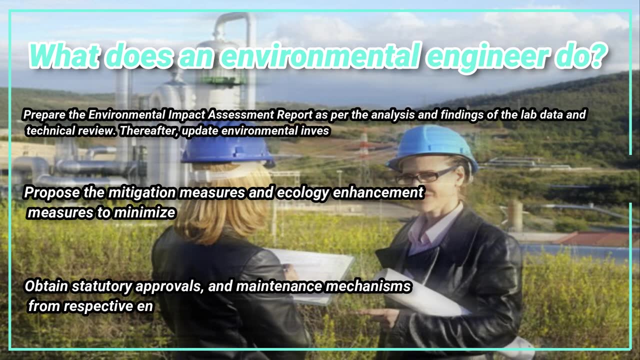 Carry out lab-based or software tool-based environment assessment of those subdomains. Prepare the Environmental Impact Assessment Report as per the analysis and findings of the lab data and technical review. Thereafter update environmental investigation reports with those assessment items, Propose the mitigation measures and ecology enhancement measures to minimize environmental 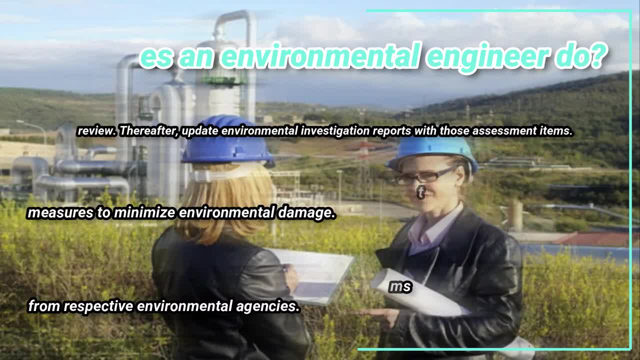 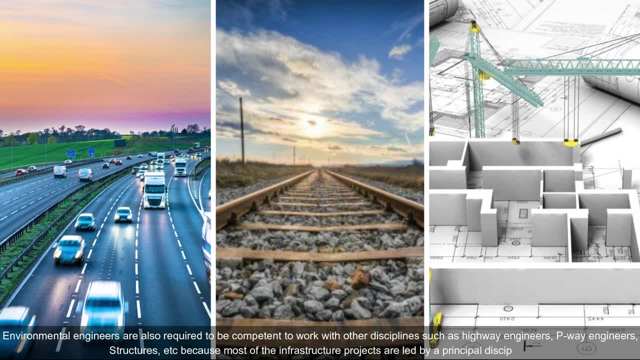 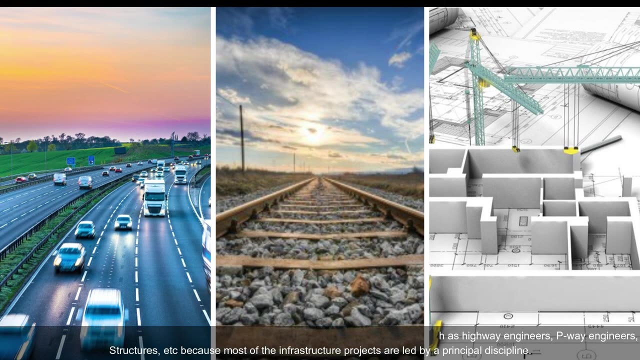 damage, Obtain statutory approvals and maintenance mechanisms from respective environmental agencies. Environmental engineers are also required to be competent to work with other disciplines, such as highway engineers, P-way engineers, structures, etc. because most of the infrastructure projects are led by a principal discipline. Educational Requirement of Environmental Engineer. 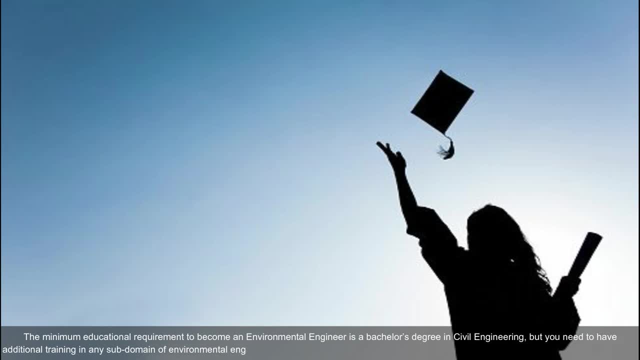 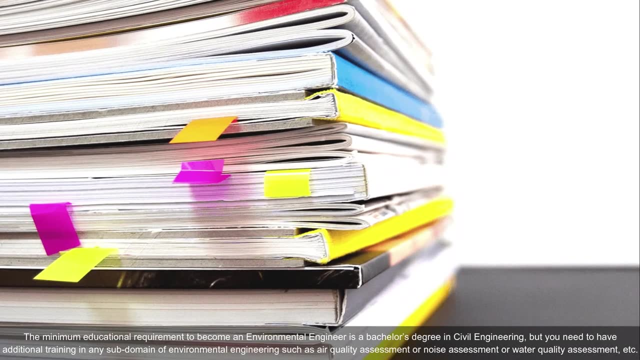 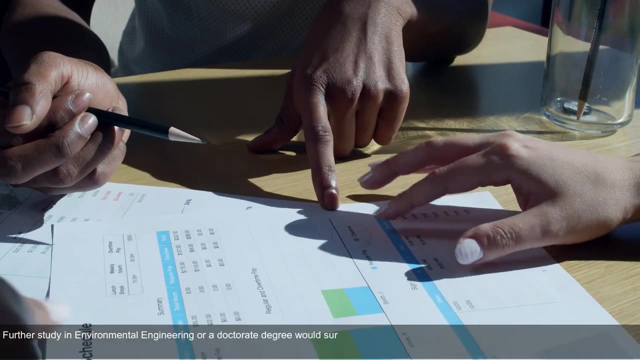 The minimum educational requirement to become an environmental engineer is a bachelor's degree in civil engineering, but you need to have additional training in any sub-domain of environmental engineering, such as air quality assessment or noise assessment or water quality assessment, etc. Further study in environmental engineering or a doctorate degree would surely. 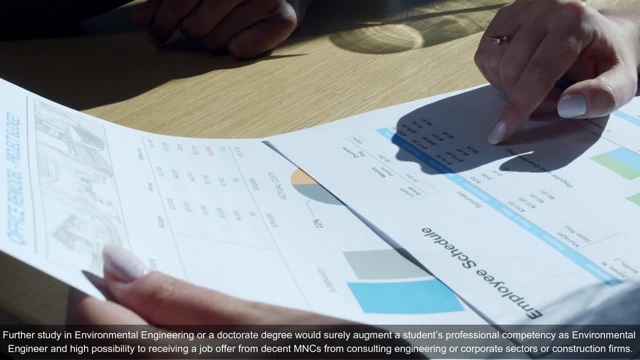 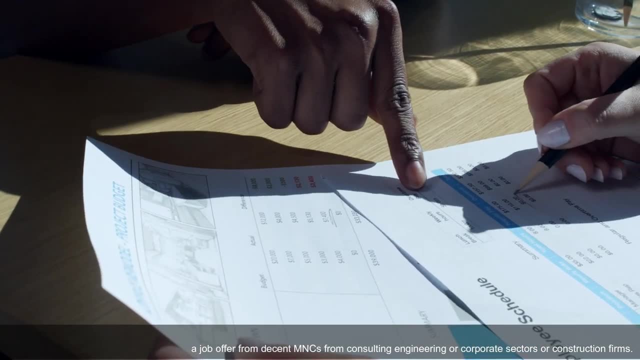 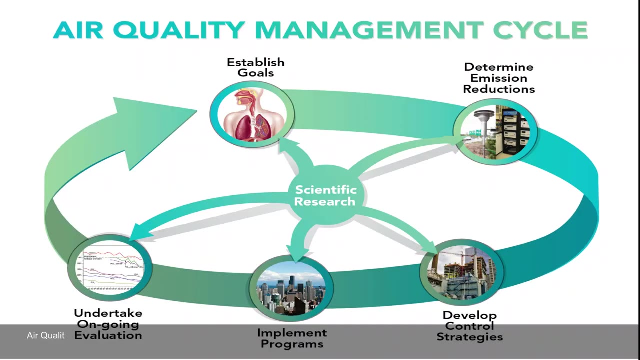 augment a student's professional competency as environmental engineer and high possibility to receiving a job offer from decent MNCS from consulting, engineering or corporate sectors or construction firms. Software Skills of Environmental Engineer. Air Quality Assessment: Air quality assessment is required for various reasons, such as compliance with planning applications, environmental implications and the like. Air quality assessment is required for various reasons, such as environmental engineering or a doctorate degree would surely augment a student's professional competency as environmental engineer and high possibility to receiving a job offer from environmental engineer and high possibility to receiving a job offer from a company. 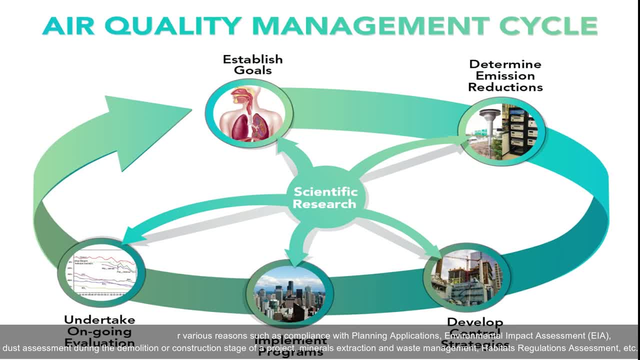 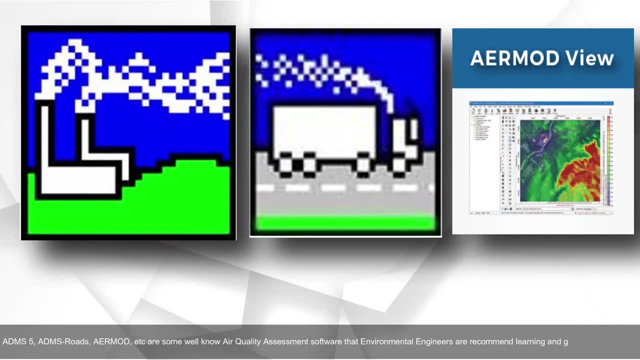 Impact Assessment, EIA, Dust assessment during the demolition or construction stage of a project, minerals extraction and waste management, habitats regulations assessment, etc. ADEMS 5, ADEMS Roads, ERMIT, etc. are some well no air quality. 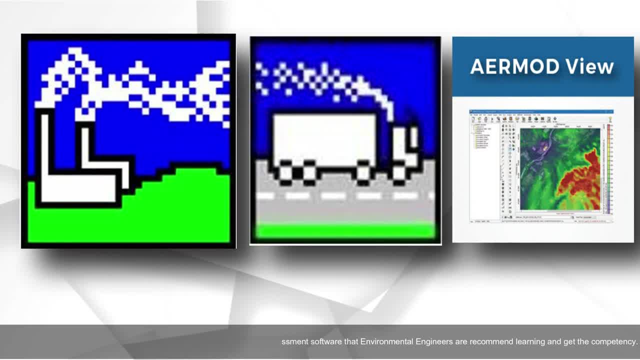 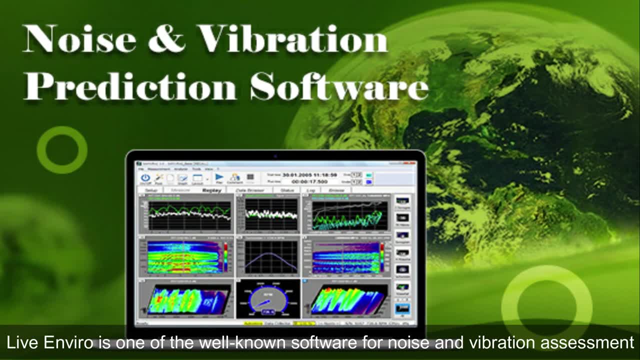 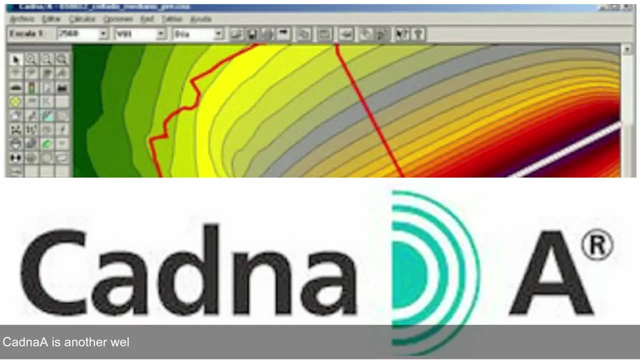 assessment software that environmental engineers are recommend learning and get the competency. Noise and Vibration Assessment. LiveEnviro is one of the well known software for noise and vibration assessment. Insul is another software tool to perform similar operations. Cadnaw is another well known software for noise calculation assessment. 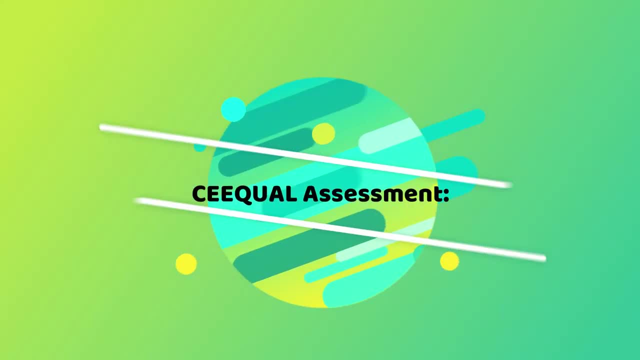 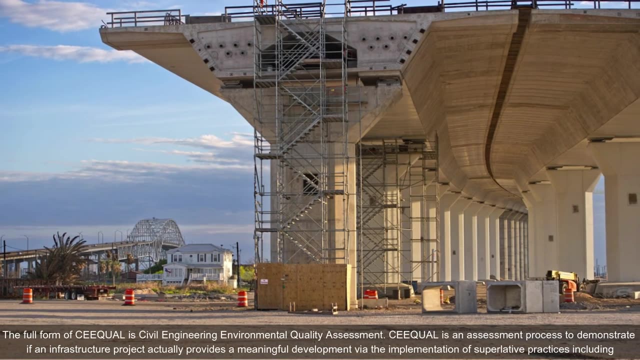 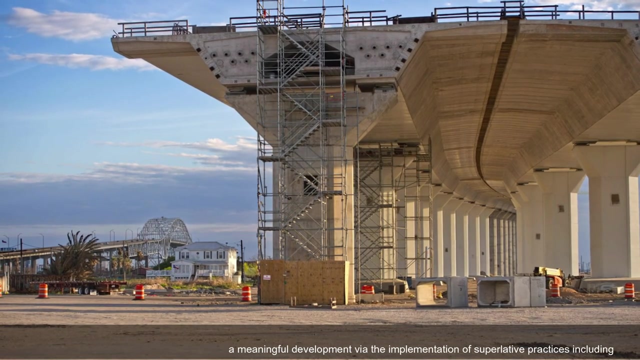 presentation and estimation purposes. Chequil Assessment- The full form of Chequil is civil engineering environmental quality assessment. Chequil is an assessment process to demonstrate if an infrastructure project actually provides a meaningful development via the implementation of superlative practices, including resource efficiency, materials, energy, water, whole life costing climate change and environmental. 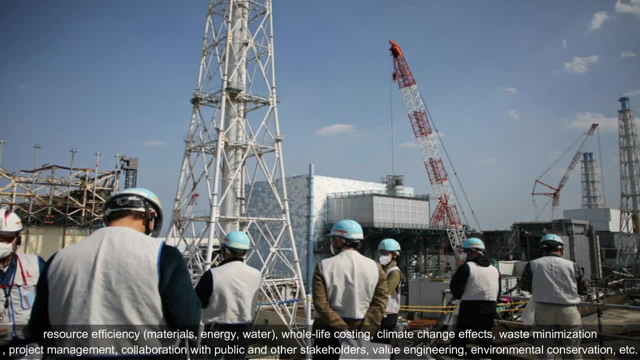 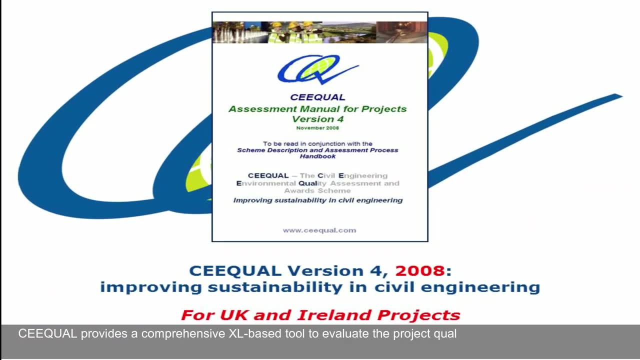 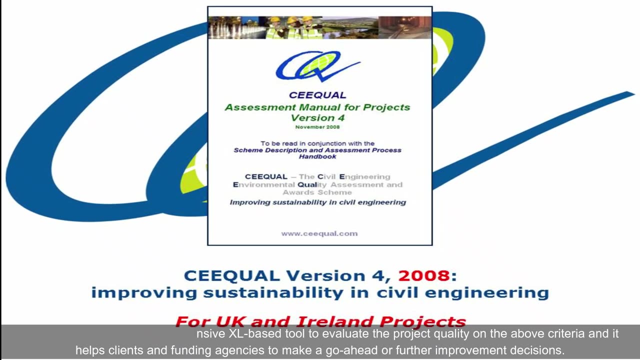 change effects, waste minimization, project management, collaboration with public and other stakeholders, value engineering, environmental conservation, etc. Chequil provides a comprehensive Excel-based tool to evaluate the project quality on the above criteria and it helps clients and funding agencies to make a go-ahead or further improvement decisions. 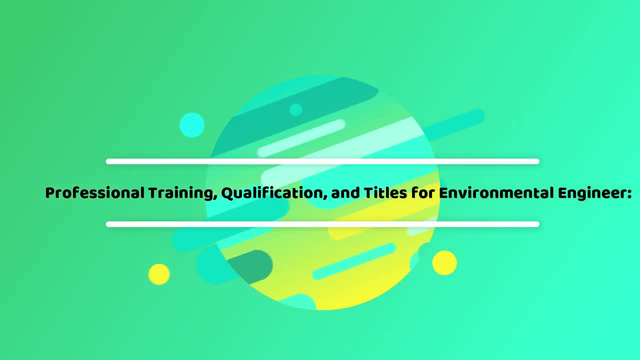 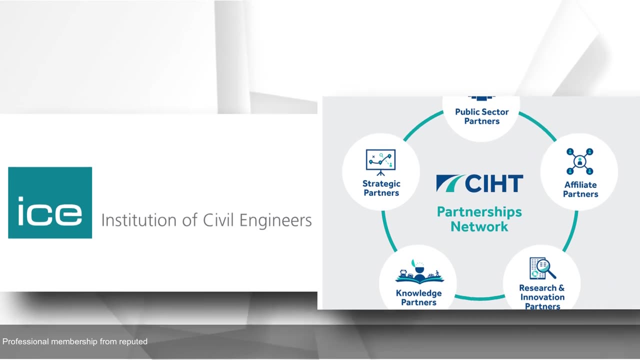 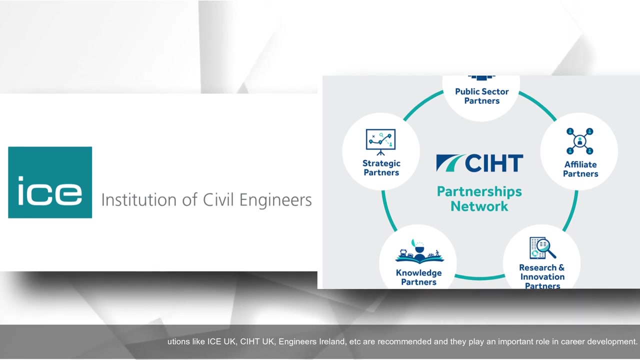 Professional Training, Qualification and Titles for Environmental Engineer. Professional training and professional titles are very important to demonstrate efficiency levels. Professional membership from reputed institutions like ICE UK, CHIT, UK Engineers Ireland, etc. are recommended and they play an important role in career. 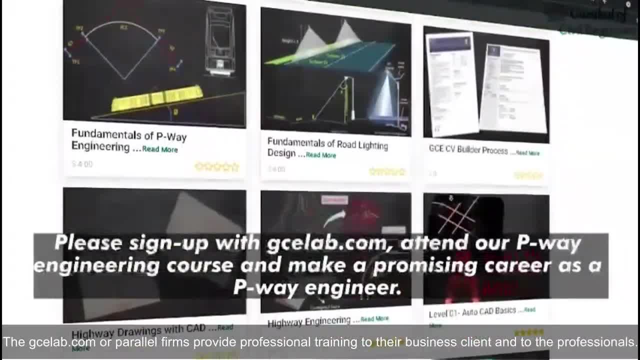 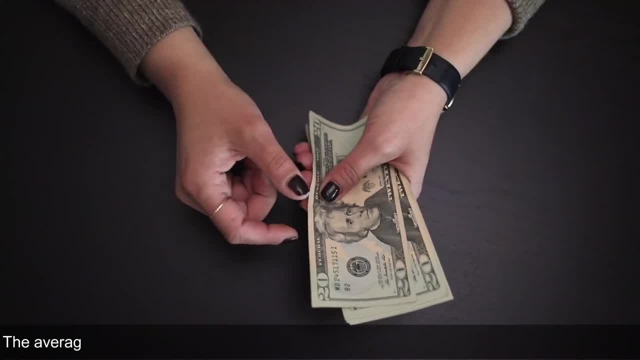 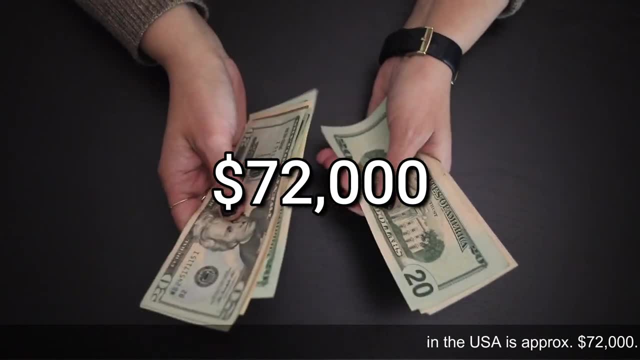 development. The G-Cell Labcom or parallel firms provide professional training to their business client and to the professionals. What is the average salary of an environmental engineer? The average salary of an entry-level environmental engineer in the USA is approx. $72,000, though. 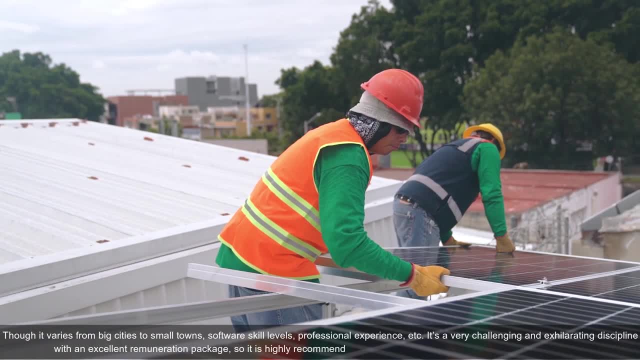 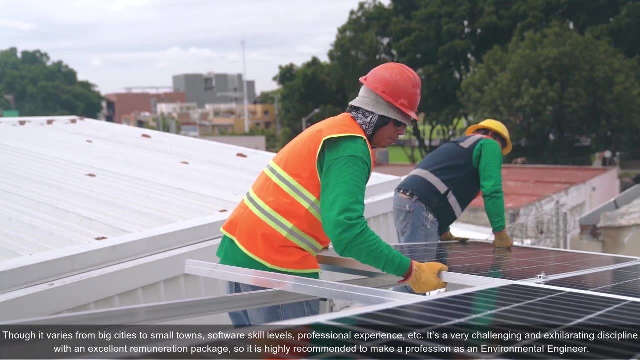 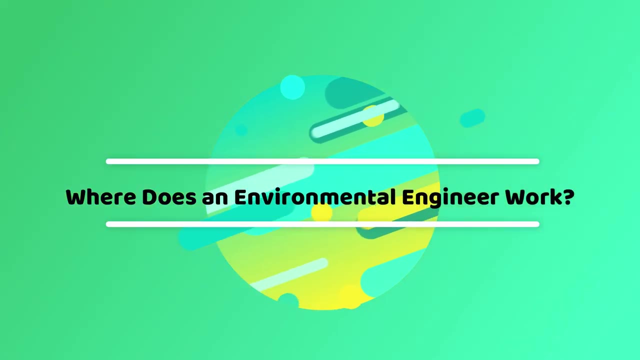 it varies from big scale cities to small towns, software skill levels, professional experience, etc. it's a very challenging and exhilarating discipline with an excellent remuneration package, so it is highly recommended to make a profession as an environmental engineer. where does an environmental engineer work? 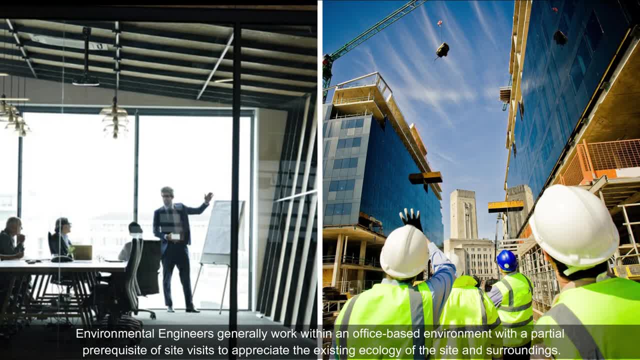 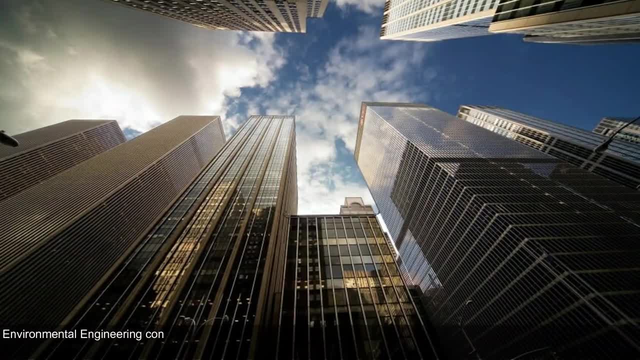 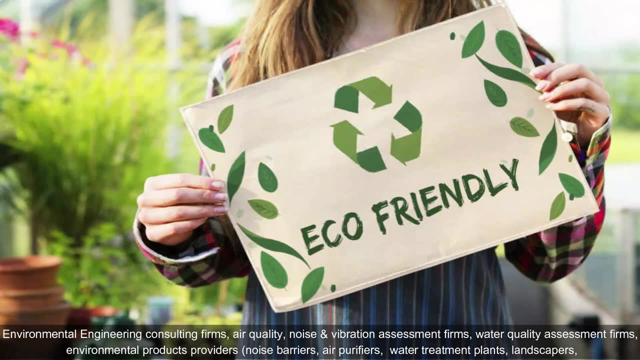 environmental engineers generally work within an office based environment, with a partial prerequisite of site visits to appreciate the existing ecology of the site and surroundings. environmental engineering consulting firms. air quality, noise and vibration assessment firms. water quality assessment firms, environmental products providers, noise barriers, air purifiers, water treatment plans. 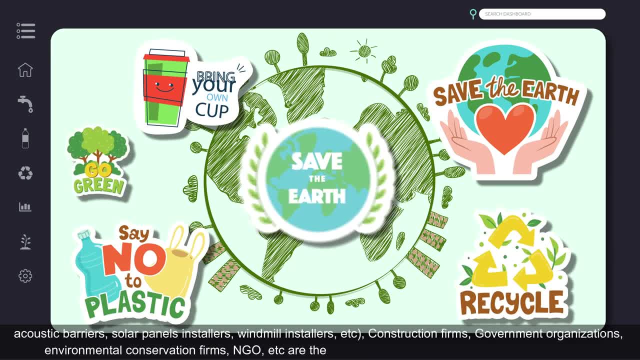 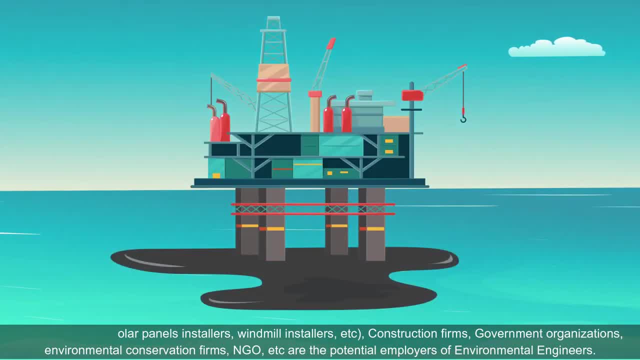 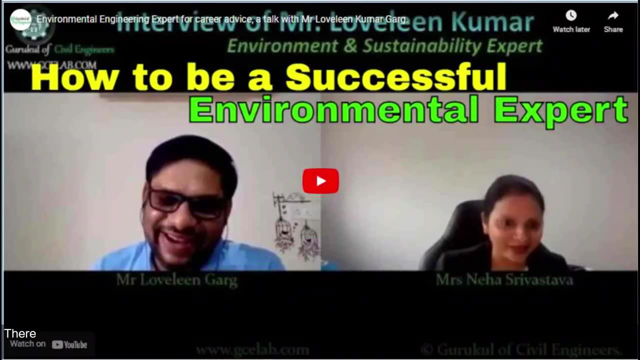 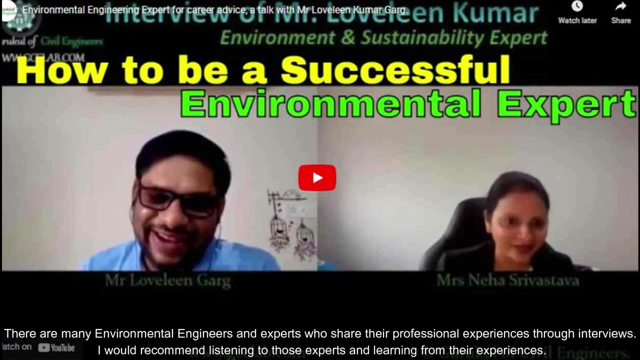 landscapers, acoustic barriers, solar panels installers, windmill installers, etc. construction firms, government organizations, environmental conservation firms and go, etc. are the potential employers of environmental engineers, interview and guidance from environmental experts. they are many environmental engineers and experts who share their professional experiences through interviews. i would recommend listening to those experts and learning from their experiences. 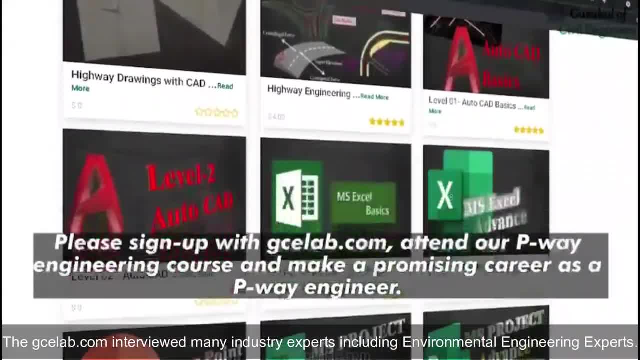 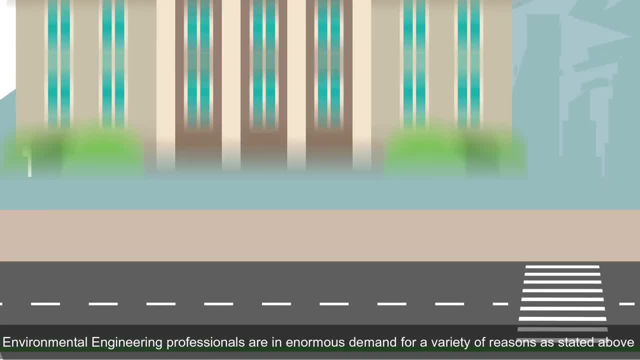 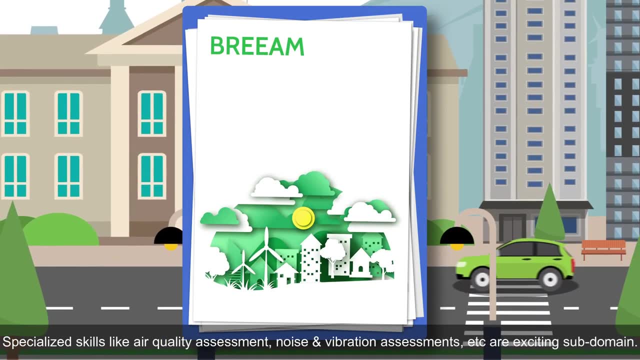 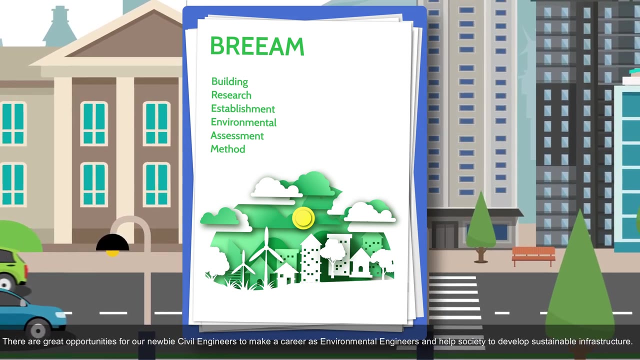 the gclavcom interviewed many industry experts, including environmental engineering expert key talkways. environmental engineering professionals are in enormous demand for a variety of reasons. as stated above, specialized skills like air quality assessment, noise and vibration assessments, etc. are exciting sub domain. there are great opportunities for our newbie civil engineers. 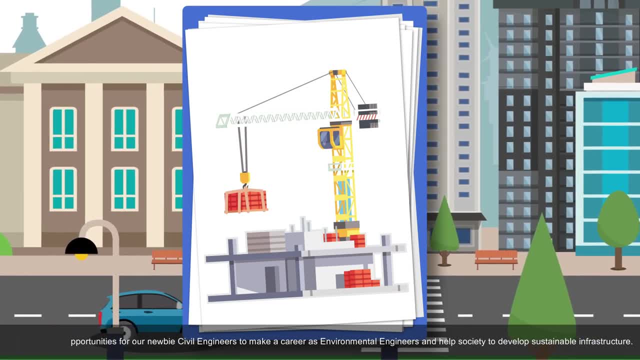 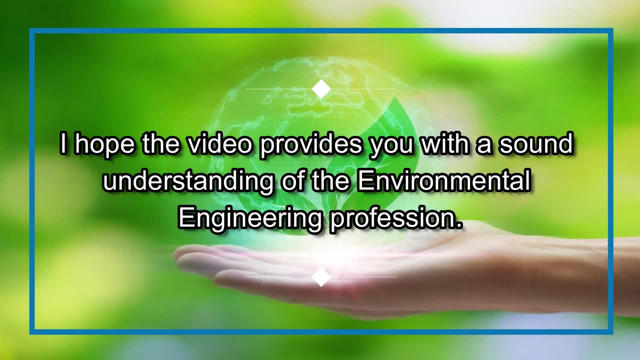 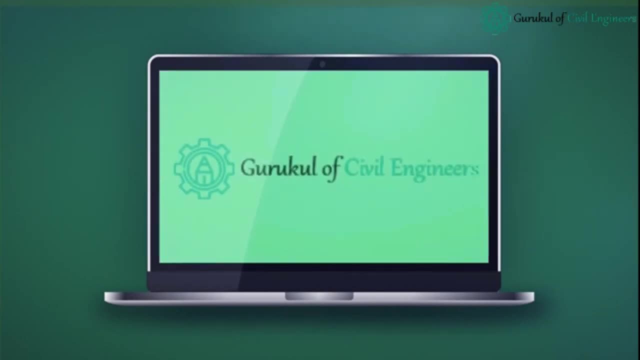 to make a career as environmental engineers and help society to develop sustainable infrastructure. i hope the video provides you with a sound understanding of the environmental engineering profession. please feel free to like, share and comment.